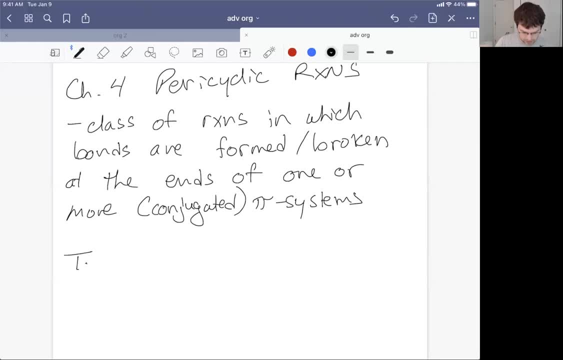 go into the types of pericyclic reactions, And so we have, at first we have- electrocyclizations, And these are. these can be either ring closures or ring opening reactions, but if we define them in the context of ring closing reactions, they could be ring closing reactions in which sigma bonds. 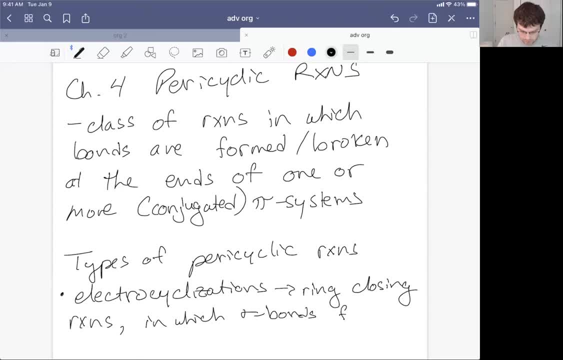 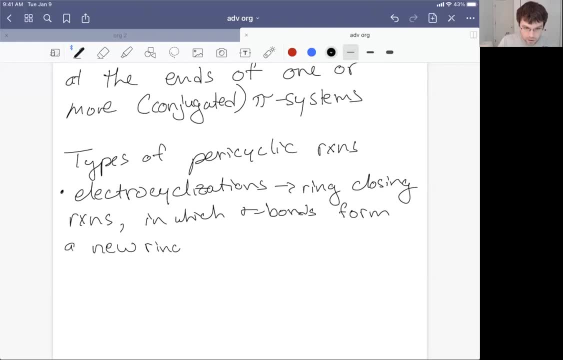 form a new ring from the end of pi bonds. Now, okay, mentally I can't think of like an exception to this rule, but there has to be like several exceptions. But I'm going to, instead of writing always, I'm going to write often. 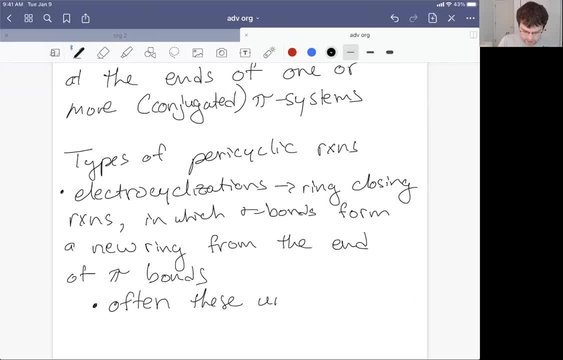 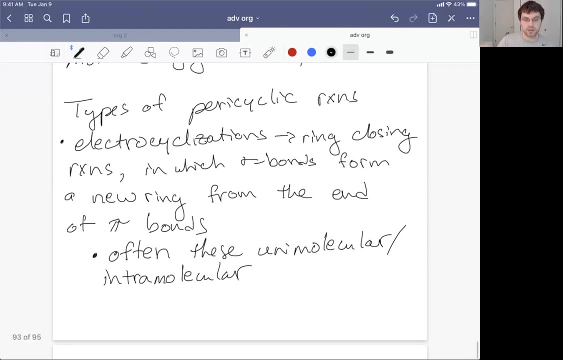 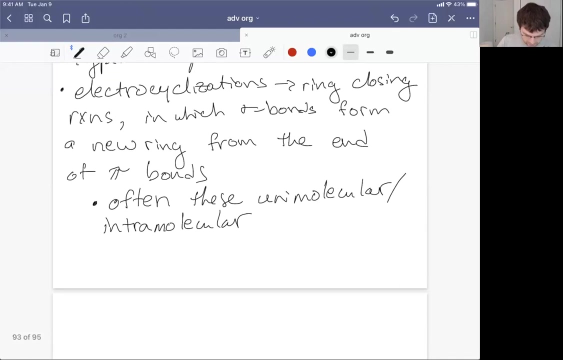 These are unimolecular reactions, And maybe another word is slash intramolecular, That is, these types of reactions occur within the molecule, so within the self of the molecule, or whatever these types of reactions occur. Okay, so there's a key driving force for these reactions before we get into several examples. 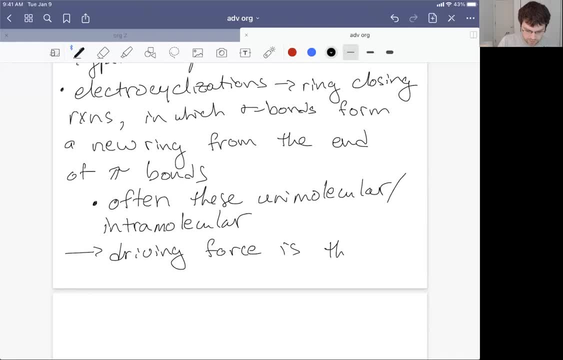 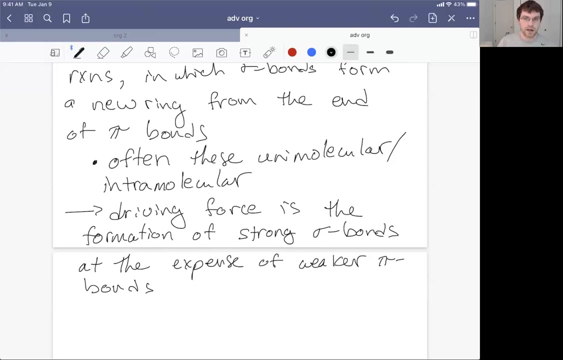 The driving force is the formation of strong sigma bonds. The formation of strong sigma bonds at the expense of weaker pi bonds. Okay, That's always an important point. The other important feature of these reactions is to think about why they go in a particular direction. and it's because the head-to-head overlap of sigma bonds is a lot more energetically favorable than the side-to-side overlap required for pi bonding. 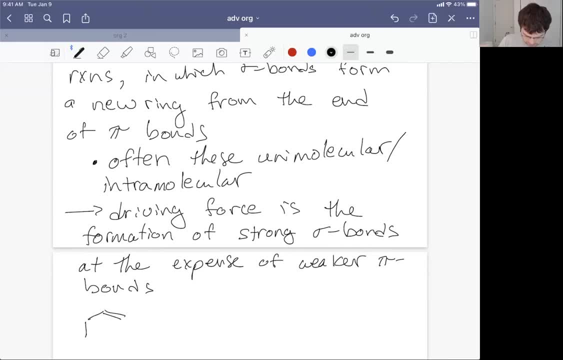 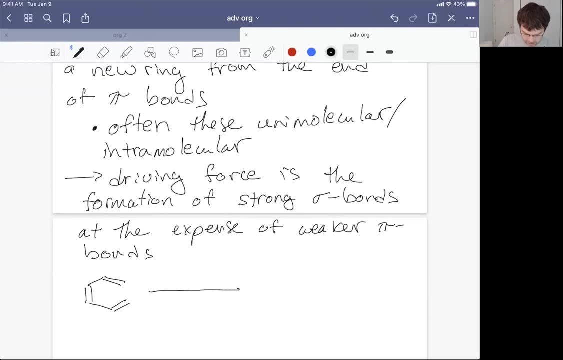 And so my favorite example is the 6-pi electrocyclic ring closure. Okay, So this looks a lot like, or is reminiscent of, a Diels-Alder reaction, but we'll look at those types of reactions here in a second. 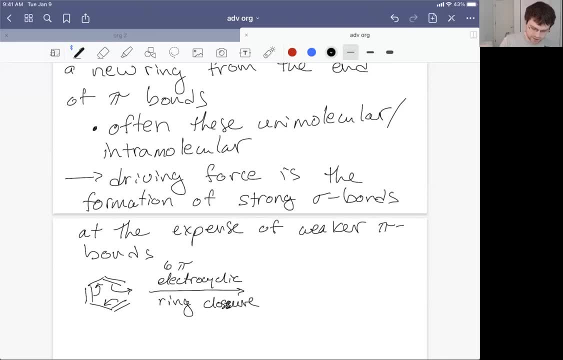 Diels-Alder reactions are different because they're not always, definitely not always, but in many cases they're bimolecular reactions And just so you're aware of the terminology, I'm going to give you a little bit of an example of a bimolecular reaction. 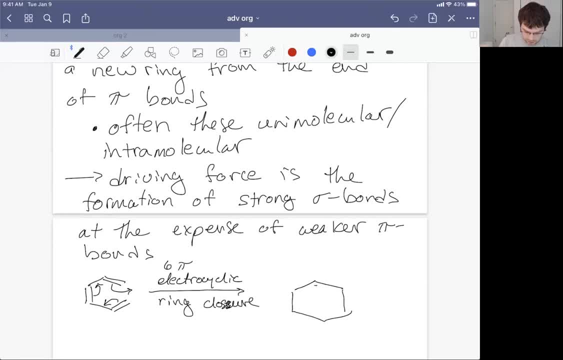 Okay, Aware of the terminology that's coming, we would call those cycloaddition reactions, which is a different word than electrocyclic reaction, And for good reason. These things are just different transformations overall and have different steric requirements. And so, if we look at this, we start with three pi bonds. 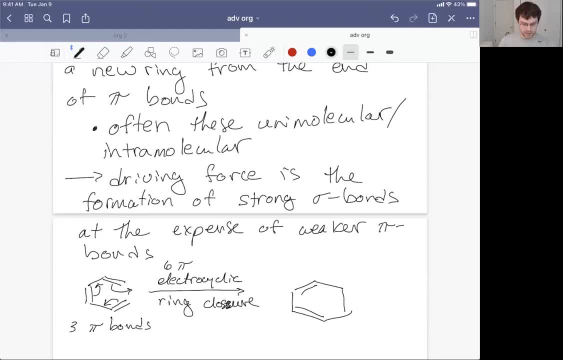 That is three second bonds between two carbon atoms, three pi bonds, and at the end of the reaction we have two pi bonds. and at the end of the reaction we have two pi bonds, pi bonds and then one sigma bond is new. so there were already several sigma bonds, but the sigma 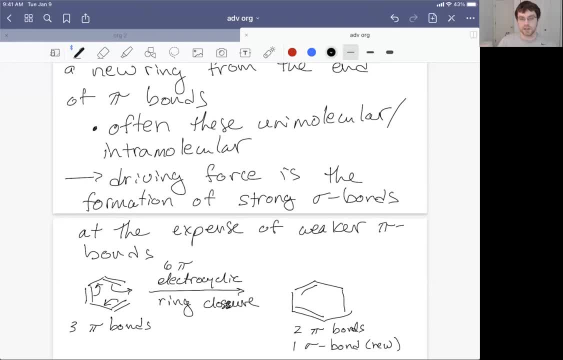 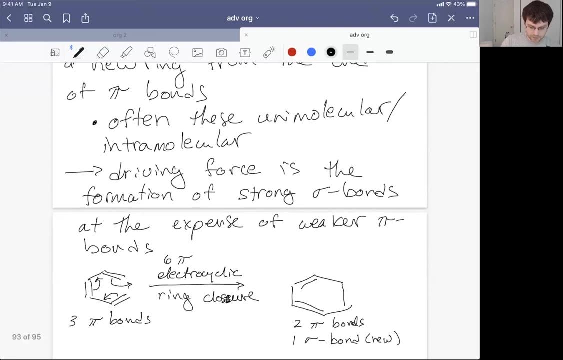 bond changes one and the pi bond changes negative one, and so you lose a pi bond. you pick up a sigma bond. this makes this an energetically favorable process, and this, this, is what allows for the reaction to actually occur, because it turns out that this is um reversible. okay, now it's i. i didn't. 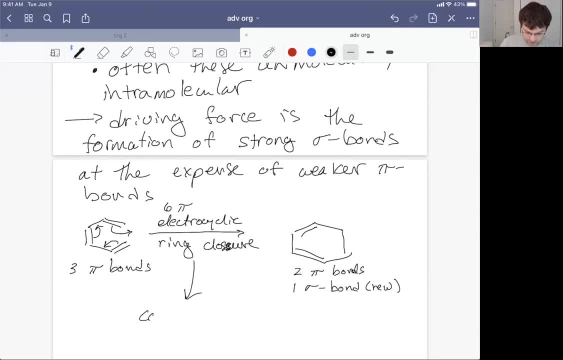 actually mention the conditions. i just wrote the name, so the conditions are heat or light for this reaction. so we write heat for the uh, um, like alchemist symbol for fire, i learned as. or also just delta energy, um, and then hv for planks, constant times. the frequency of a photon gives. 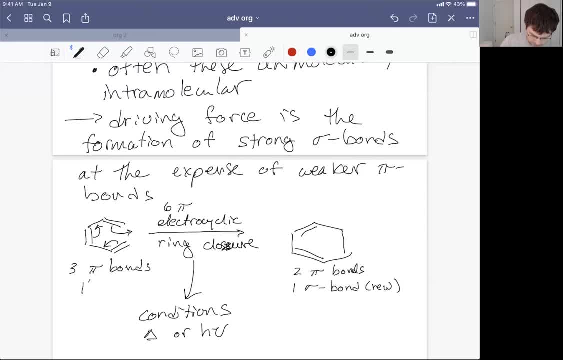 you some energy of a photon. so that's how we supply our energy now. three pi bonds, which i labeled in the outset, means we have three times two equals six pi electrons, because we like to think of there being two pi electrons per second bond between two atoms. okay, so this is an electrocyclic ring closure, because we form a ring. so a new ring has formed. there could also be electrocyclic energy. so we have three times two equals six pi electrons, because we like to think of there being. three times two equals six pi electrons, because we like to think of there being. now it turns out if you take a cyclobutene. 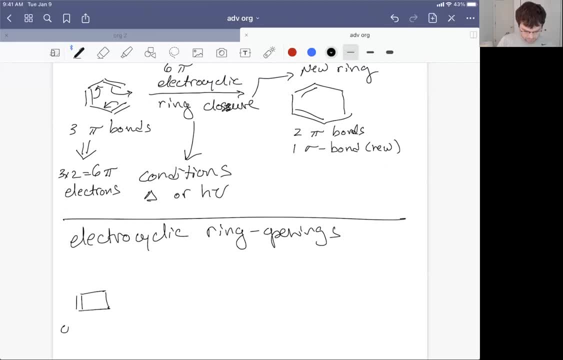 okay, and you expose this to either heat or light, you will get a. you'll get a cyclobutene- right the name down here: a four pi electro cyclic. right the name down here: a four pi electro cyclic. right the name down here: a four pi electro cyclic. 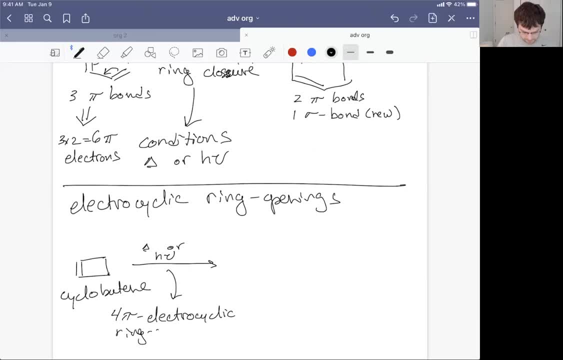 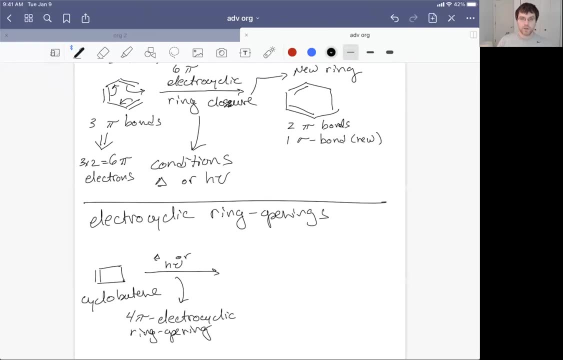 ring opening, ring opening. now what that looks like is we're actually going to now. what that looks like is we're actually going to move in the opposite direction that we did previously. so previously we showed we kind of rolled the conjugated double bonds around to make a new sigma. 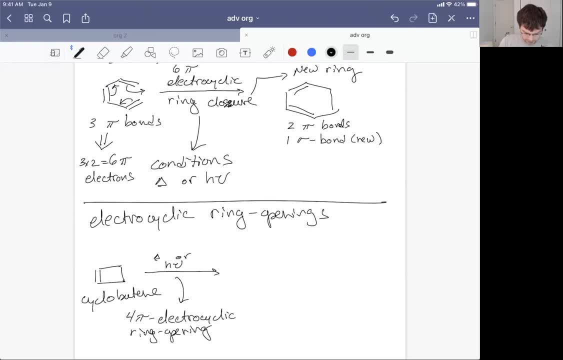 bond and then move the double bonds. here we're going to break. they start this- a sigma bond that's across from the double bonds and we get- and by break it I mean we're going to shove it down to make a new carbon-carbon double bond. 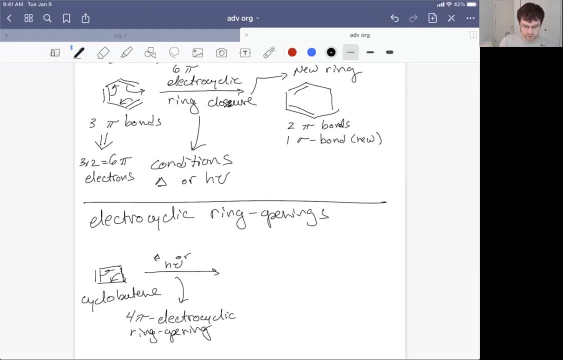 and then shove this double bond up to make a new carbon-carbon double bond up. this way, This gives us this structure, which is now a conjugated pi system. but we've lost the ring. I'm gonna just let this relax. let the geometry sort of flatten out. 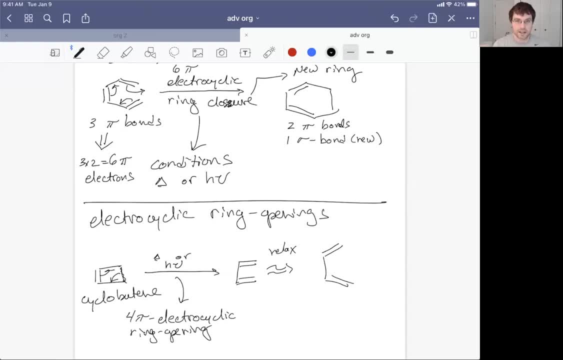 and we get a diene. remember The old saying: like help me, I'm diene, right? So anyway, everybody loves that joke. Okay, so what we've done here is we've taken a mono alkene and rolled the double bond around. 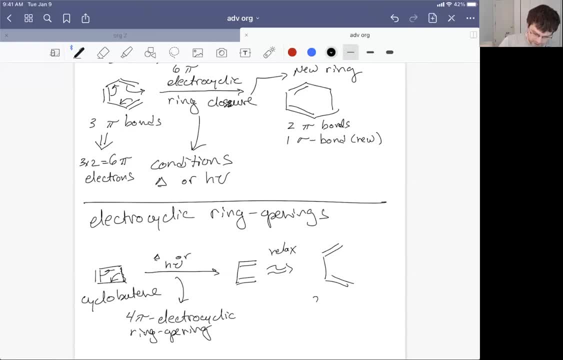 and then broke a sigma bond to give rise to two new pi bonds- Pi bonds- whereas before we lost one sigma bond. And actually it's not two new, it's one new pi bond, excuse me. So here we exchange a sigma bond for a pi bond. 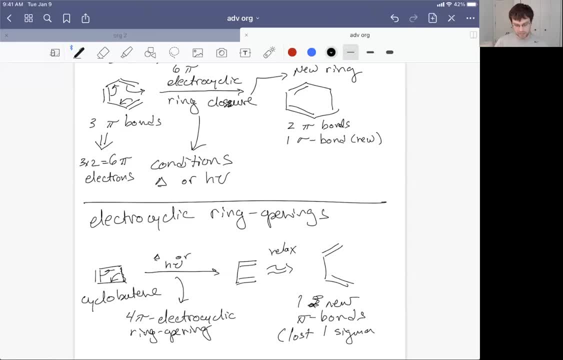 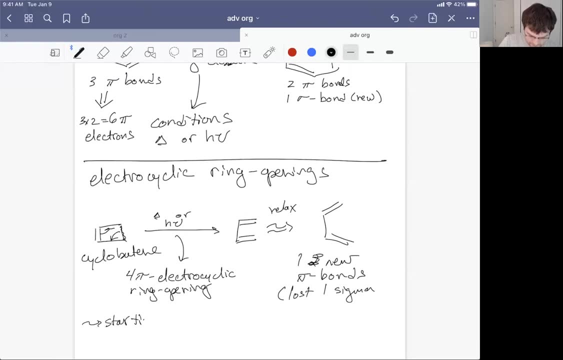 Now, why would we want to do this? The driving force doesn't seem to add up because pi bonds are weaker than sigma bonds. Well, if we look at the starting molecule, we would say the starting molecule possessed ring strain, So we had some strain and some instability built. 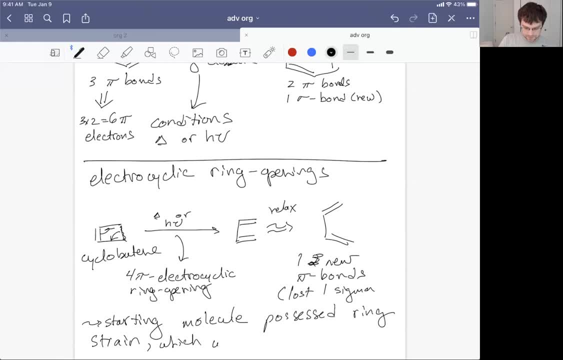 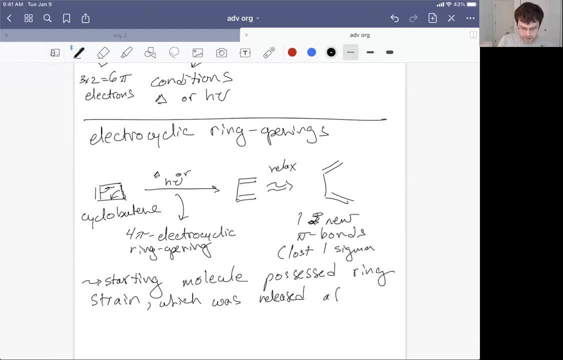 into the molecule which was released, which was released after the ring opening reaction. Okay, so those are electrocyclic ring closures, where we form a ring and then electrocyclic ring closures and then electrocyclic ring opening. That second example was when we actually opened up the ring. 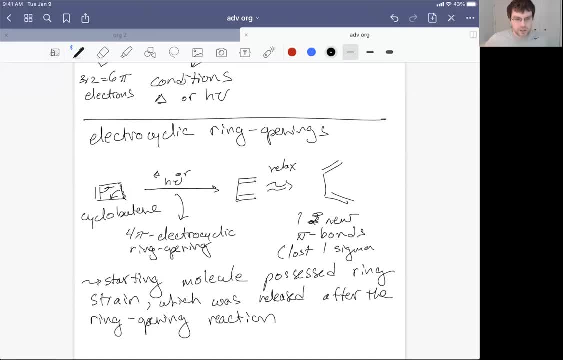 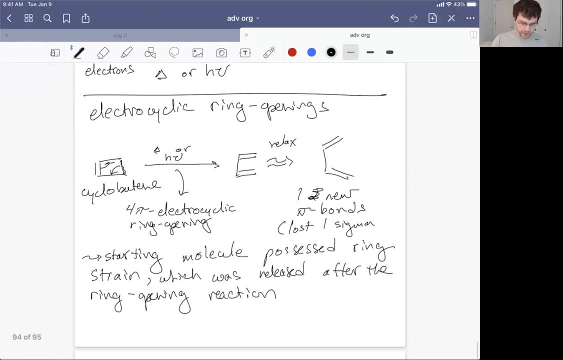 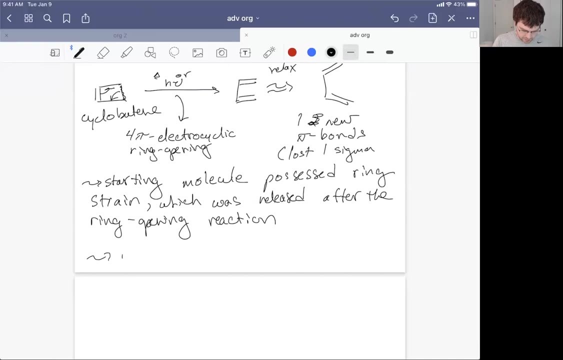 Now it's important to note that these processes can actually occur in reverse of each other. So if you really wanted to excuse me, if you really wanted to, and let's make note of that. So ring opening and ring closing reactions are the reverse of each other. 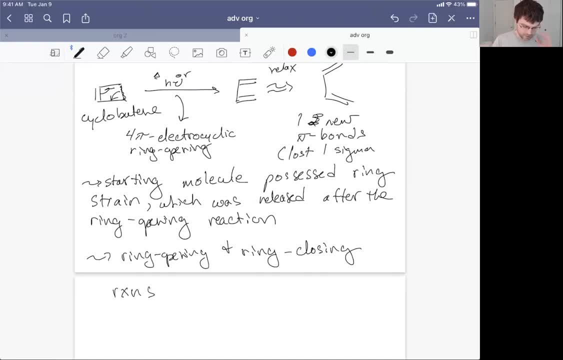 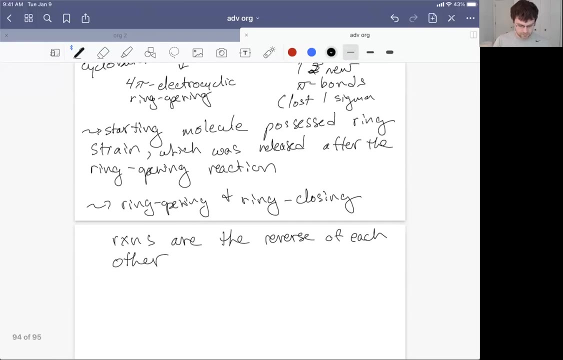 And I should have qualified this as saying electrocyclic ring opening and ring closing reactions are the reverse of each other. Okay, kind of an interesting equilibrium that we can observe is if we actually start. I just gave away the punch line. I gave away the punch line of the joke, but let's. 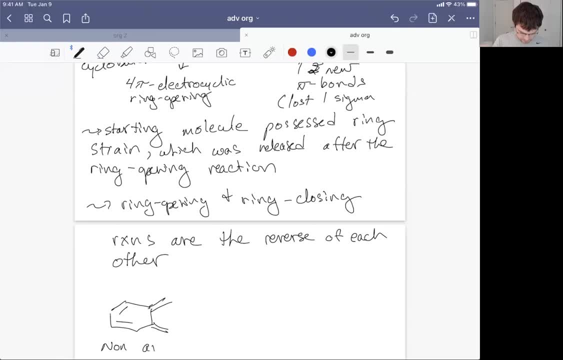 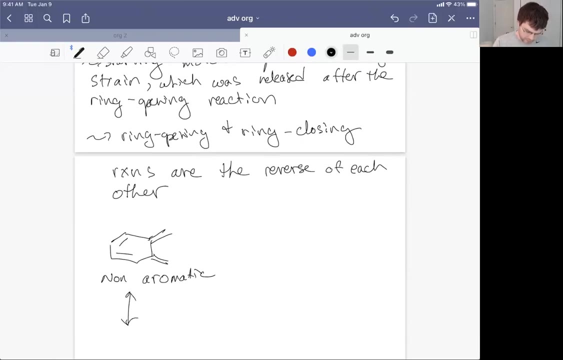 let's start with this non-aromatic molecule. It might actually be aromatic if I consider a resonance structure. I should know that before I start recording the lecture, but I think I'm already five minutes in, So I'll have to look that up after the fact. 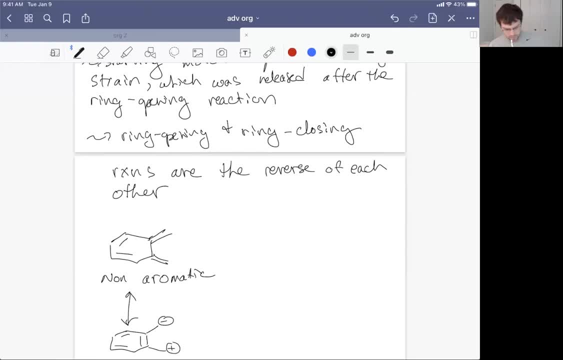 because we could consider a resonance structure like this and then it'd be a permanent dipole. it's kind of a permanent dipole to induce aromaticity. I'm gonna cross this out. Anyway, if we apply heat to this, I actually don't know where the equilibrium constant lies. 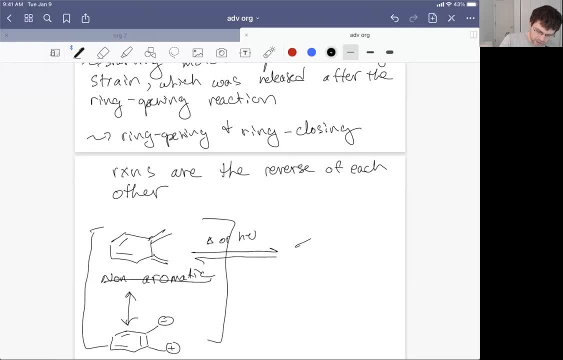 heat or light. we can actually flip back and forth between this and the cyclobutene structure, And then perhaps you want to see the curly arrows drawn this way, or you can have the curly arrows drawn this way. we have resonance structures we can get to. 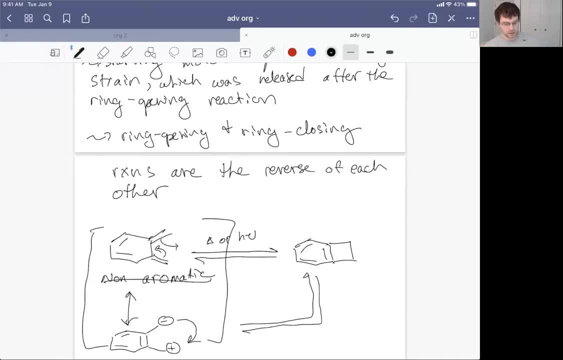 any product from any resonance depiction of a molecule. okay, so the point here is: we could, we could do ring closing and ring opening reactions, or just the reverse of each other. if you can go one way, you conceivably can go the other way. now this one's a really interesting 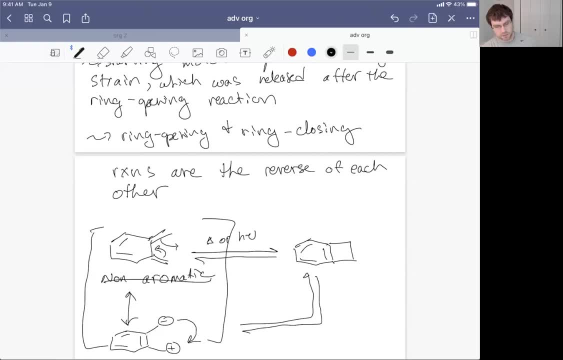 equilibrium because it's got a driving force towards less ring strain. but less ring strain but a permanent dipole to get to aromaticity or no aromaticity, which isn't a good situation, or you could absorb that ring strain, deal with it and get to a permanently aromatic molecule. 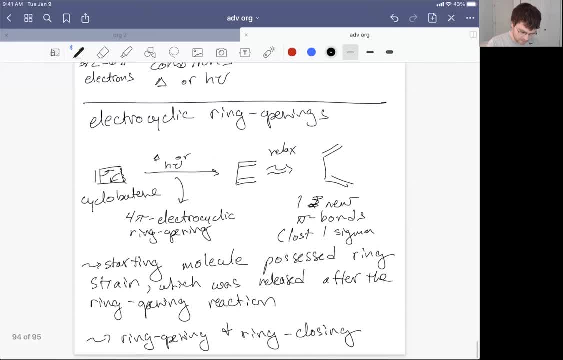 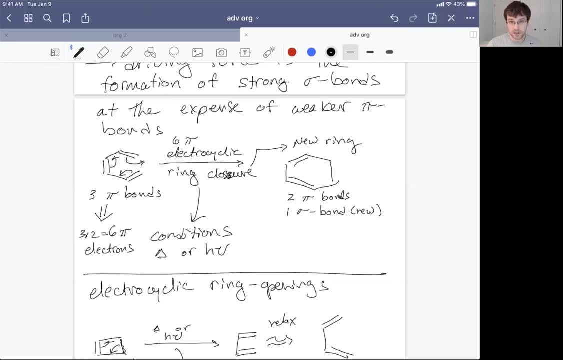 although we have some kind of twisted bonds in there. yeah, it's a really interesting molecule. okay, what I want to do is take a second and just go back to the six pi electrocyclization, so we could consider the reverse of that if we wanted to. 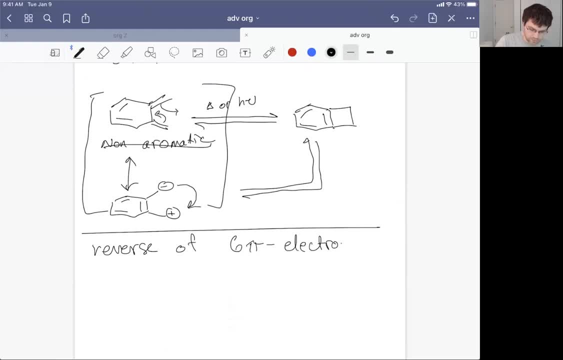 so the reverse of the six pi electrocyclic electrocyclization would be where we start with the ring closed product and then we move the bonds around. now that's not a super favorable process because we're not alleviating ring strain to do the electrocyclic ring opening and we're building in a new pi bond. 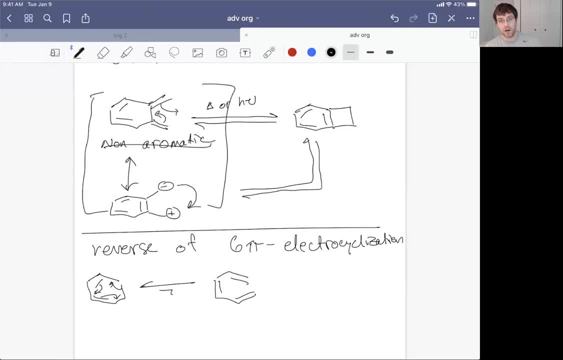 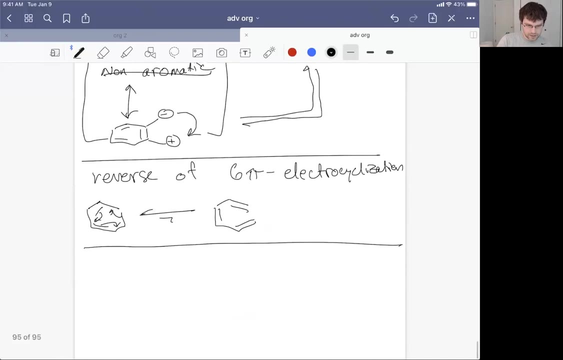 but you can draw the arrows there if you need to. so maybe they're something else to offset that energetic cost and perhaps drive the reaction towards the product, which would be kind of interesting. so ring opening, ring closing reactions work together. now these things can get kind of um, these things can get kind of funky in in some ways. i'll just 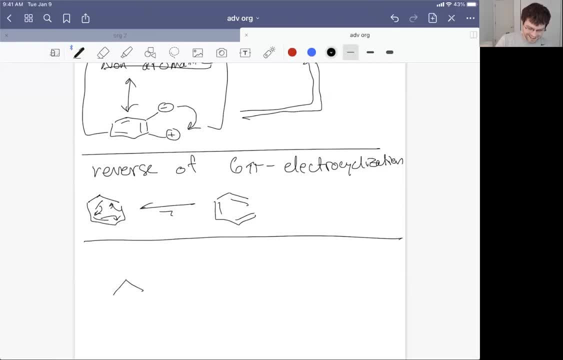 i'm going to leave that description there and i'll go on the record as calling some chemistry funky. so what i want to do is consider this cyclopropanone substrate. so it's just a cyclopropane with a carbonyl, and cyclopropanes are weird but they're not uncommon, and if you 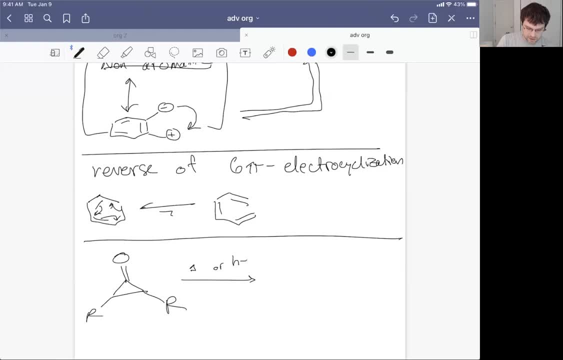 apply heat or light to this. you can actually access what's called the dipolar intermediate, where you've got this enolate structure, and you can actually apply heat or light to this. and you can actually apply heat or light to this next to a carbocation. now, how did that form? well, there's a few ways that you could think about forming this product. 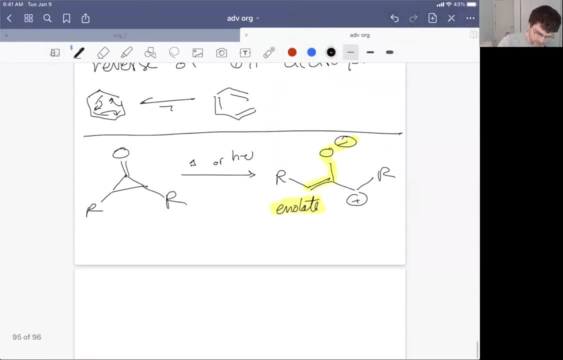 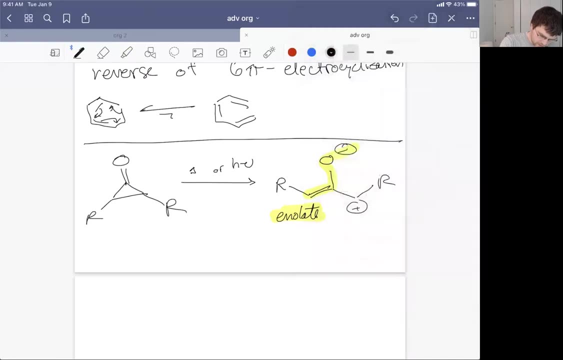 looks like i need to build some paper. you're sorry. let's see if i can add the pages without freaking out. there we go, okay, sorry about that. okay, what we could do is we could consider a resonance structure of this where we've got the carbonyl separated as a negative on oxygen, a positive on carbon, and then all we have to do 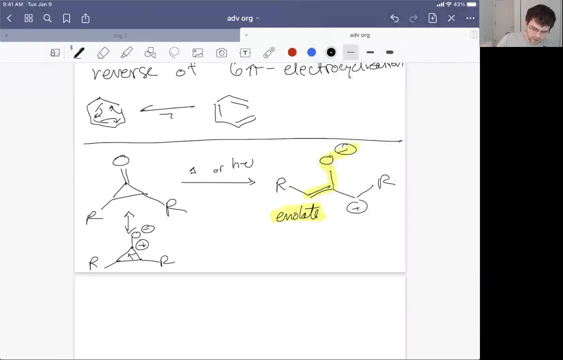 is just shove one of the bonds over to make a carbon carbon double bond and leave behind a positive charge, which would be at this position, and i'm not sure if you can trap that, that bond, that dipole, you can actually push this intermediate or this equilibrium towards the product. so that's. 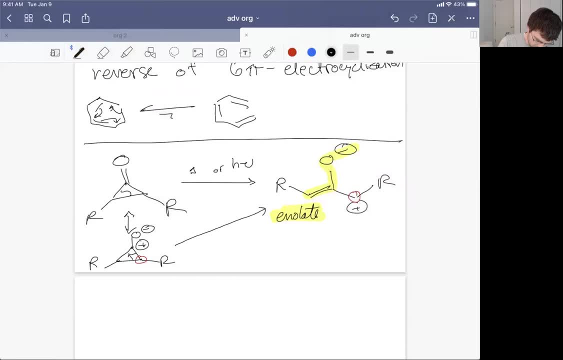 one way to draw it and, alternatively, what you could do is you could go from here to here to give rise to the product. remember, any resonance depiction can get to the product. resonance depictions are depictions of the same molecule. if you do a good job drawing resonance structures, you can actually 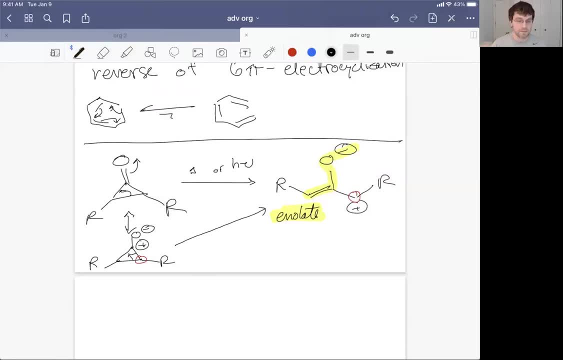 get to any product. any resonance structure can get to any product. that's my point. okay, if you have questions about that, let me know. okay, so these things can get kind of interesting. i don't know, maybe we call this a, a, two pi, electrocyclic ring opening. it's kind of. 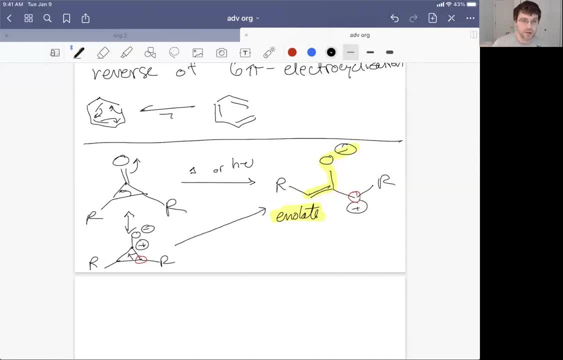 interesting, but anyway. so those are electrocyclization reactions and they they come in a lot of different flavors with a lot of different electron counts, and from organic chemistry too. this is where you use the thumb trick to think about conrotatory and dysrotatory ring opening. 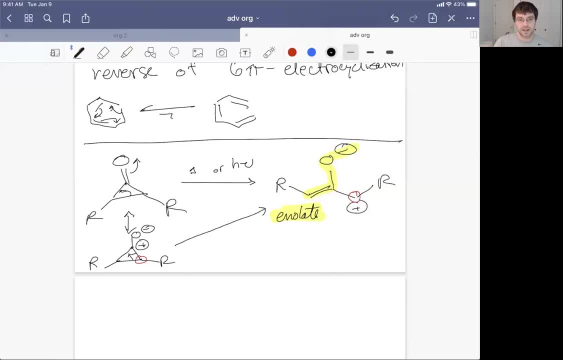 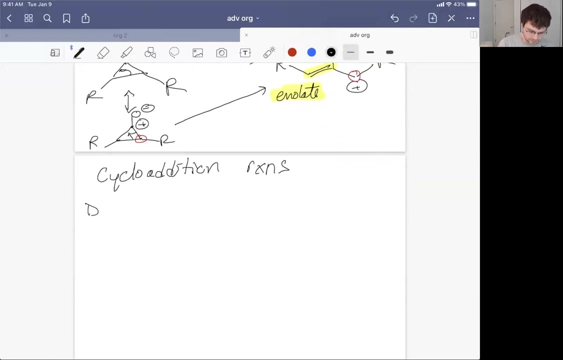 to predict stereochemistry, the product: there's a nice section in the textbook on that. next we're going to go into cycloaddition reactions and by far my favorite cycloaddition reaction is the diels-alder reaction. but it's not the only cycloaddition. let's get that out there, the diels-alder cycloaddition. 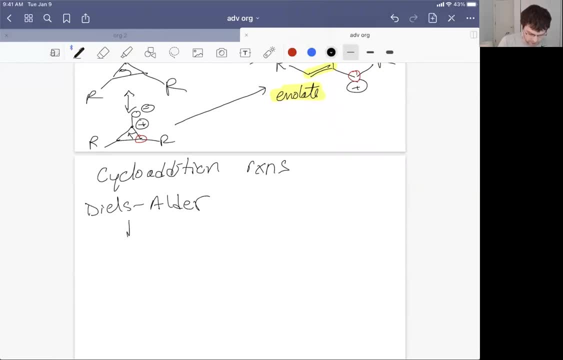 so in the diels-alder cycloaddition reaction what we do is we first of all call this a four plus two and those go in brackets, for some reason, cycloaddition reaction. so in the four plus two cycloaddition reaction we take a diene. 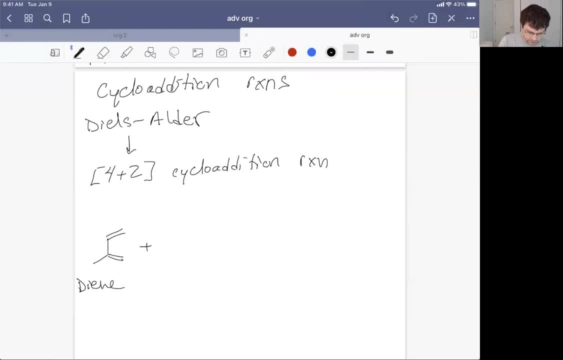 and we add it to a, an alkene, an alkene that we label as the diene reaction, and we add it to an alkene reaction and we add it to an alkene reaction. so this word becomes 1 and if you look at the cycle and the on, that really tells us. 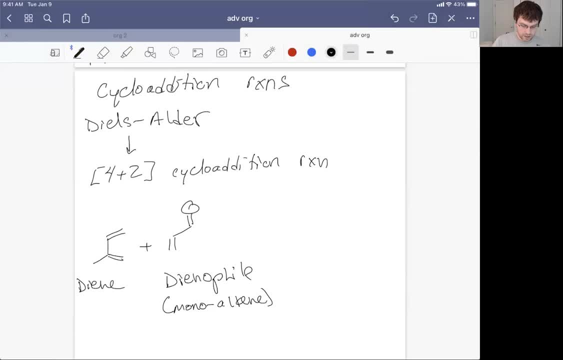 that thissmith used this, getting used to the process and just looking at the transformation decision here, we find that the newje and to drive down the cell die in aelia ago now. on the other hand, if we look back over the deadly on sticks, 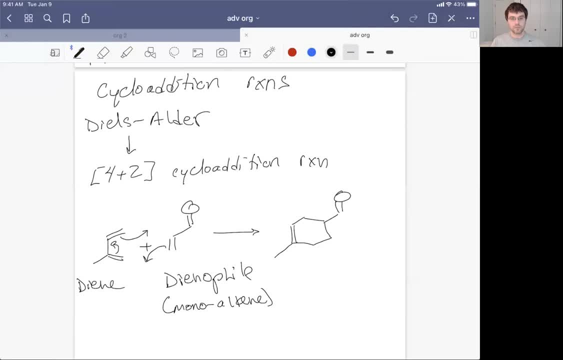 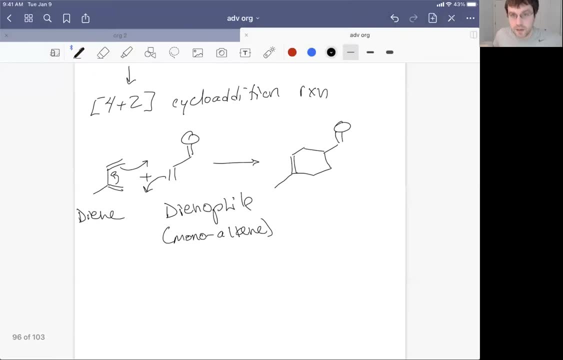 if we're working after some healthy evaluations of the die, you know, file telling us that that is the alkyne, that is the molecule that possesses the pi bond it's going to react with. Okay, Now, what's important to note is that I could have the orientation of the diene or the dienophile sort of flipped in this case, because I don't have a symmetric diene and dienophile. 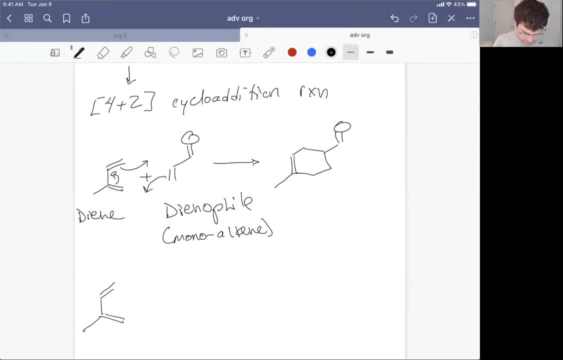 That is to say, I could go here, I'm going to leave the diene alone, but I'm going to rotate the dienophile such that now We have the carbonyl now closer to the methyl group. Now what's important to note is that these two structures are isomers of each other, and I would classify them as what's called a regioisomer, because these two structures have sort of reacted at different sites or regions of the molecule. 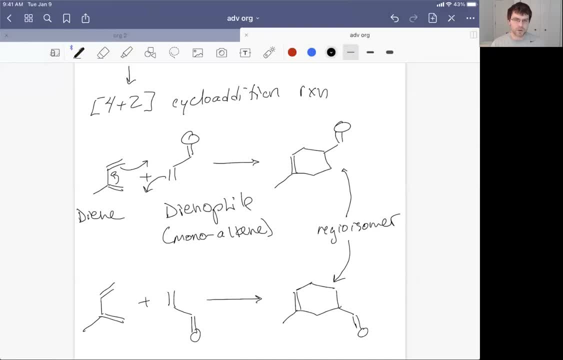 Okay, And the regioisomer word works really well if you have multiple types of the same type of functional group present, but it's harder to understand here. But what we say here is that we're reacting with different, I guess, orientations of the p-orbitals that have to overlap, if you remember all of those perspective drawings. 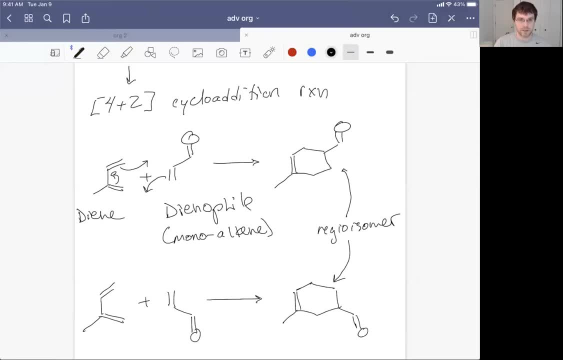 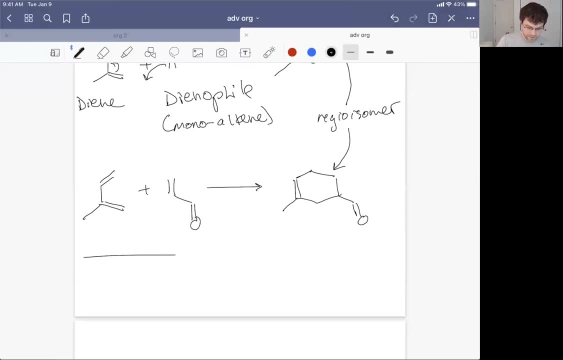 Anyway, I could belabor that point probably too much and hit diminishing returns quickly. So Let's go ahead and look at some examples that are sort of fun. So I think this is a fun example. We're going to pick on the same diene structure that we had earlier or, excuse me, the same polyene structure that we had earlier. 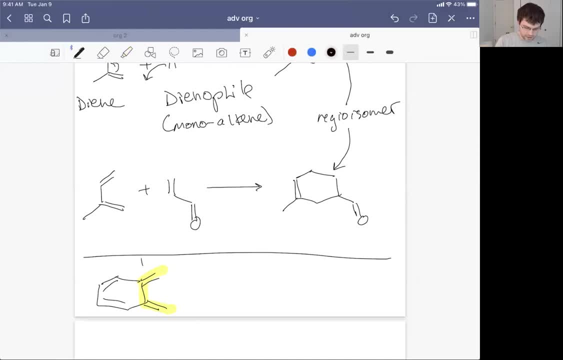 And I'm going to focus on this part- to be the diene. Now, there's actually- it actually sort of looks like there's two dienes present, but this one is the more reactive pair of pi bonds because if it finds a monoene, I'm going to label this diene in yellow. 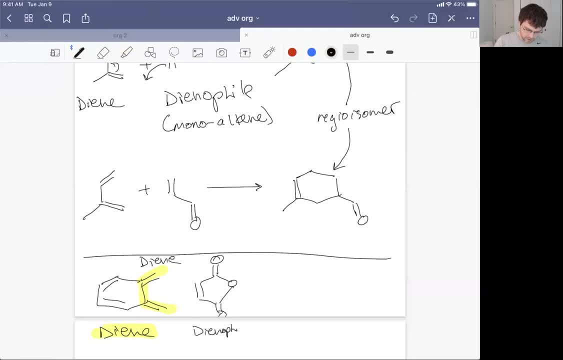 And I'm going to label this dienophile in a different color. So we're going to react with this pi bond And if we do the 4 plus 2 cycloaddition here, we actually generate an aromatic benzene ring in our product. 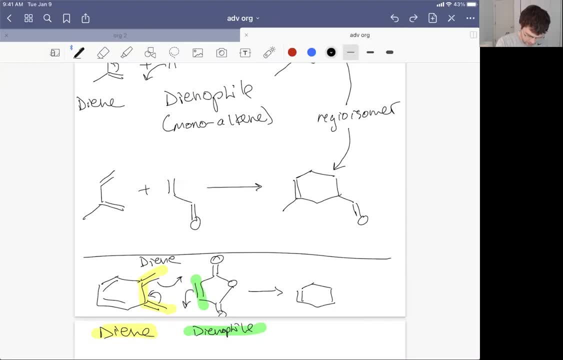 I don't want to rotate those, I want to be careful about my double bonds. so you guys can see this. It does not matter though. So we actually form three rings in the product. if you want I can, I can trace the various bonds. So here were the carbon atoms involved in the dienophile structure. 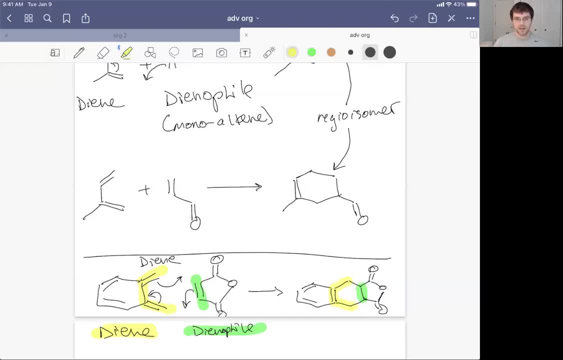 And then in yellow, here are the carbon atoms present from the product. And then in yellow, here are the carbon atoms present from the product. here are the carbon atoms involved in the diene structure. So it's pretty cool, because you generate an aromatic ring during the course of the Diels-Alder reaction. 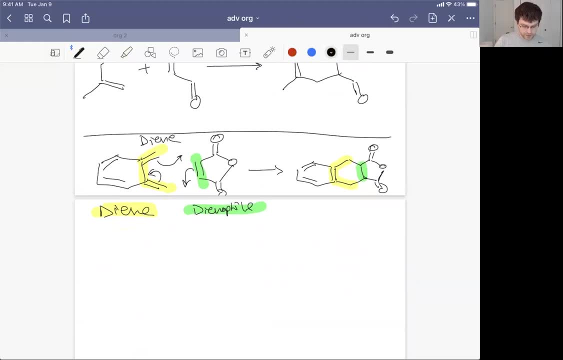 Now let's look at an example where we actually, instead of picking a typical diene dienophile, we could pick a diene Okay so or, excuse me, an alkyne to be the dienophile. Let me say that, again, I'm replacing the dienophile, which is just a monoene in many 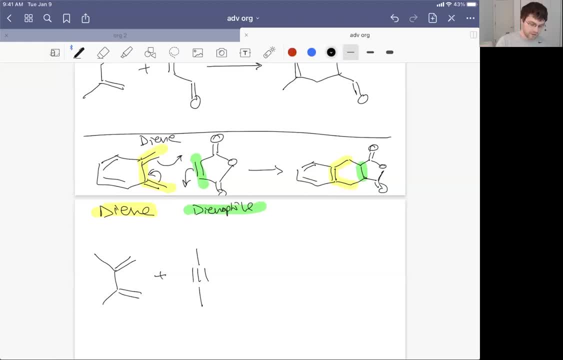 cases with an alkyne. I've added another site of unsaturation. I've added another double bond present. Okay, so here's my diene. Hopefully you can see that clearly. And then here is my dienophile, one of those pi bonds on the triple bond. The other one is unreactive under these. 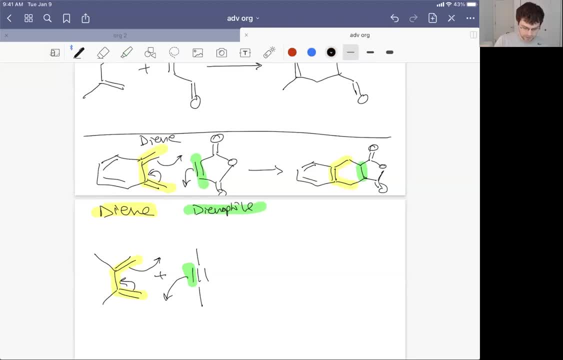 conditions and won't engage with the diene. And what that results in is, you know, a six-membered ring with one double bond here, which is part of the diene, And we should attach the methyl groups. And then we have CH3s here and here Maybe I should have picked different groups. 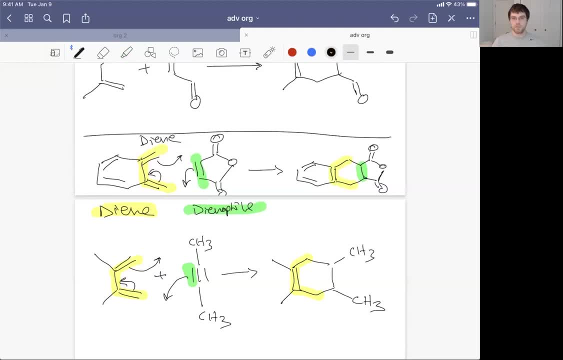 They're going to be right here and right here Now. typically, if we used a typical dienophile, we would be done, But because we used an alkyne, we still have a pi bond left over between the two dienophiles. Let's make that green, which means we have another double bond right here. So we have. 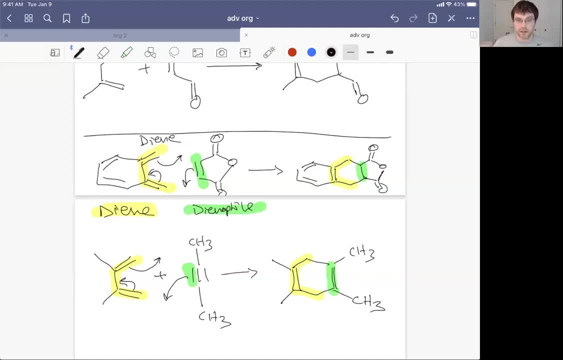 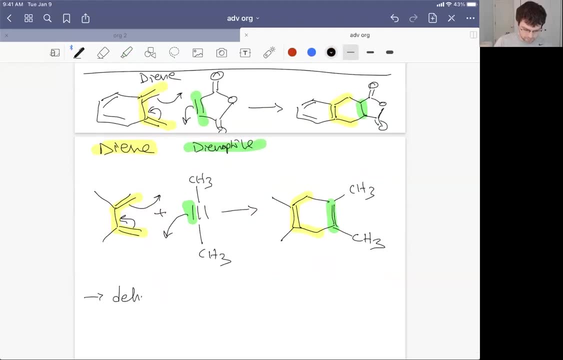 two double bonds in the products because we've included an alkyne. This is what we call a dehydrodeals alder reaction, And that's because one reactant, we say, has lost two H-atoms, And in fact, something I studied in grad school that was actually a lot of fun- was 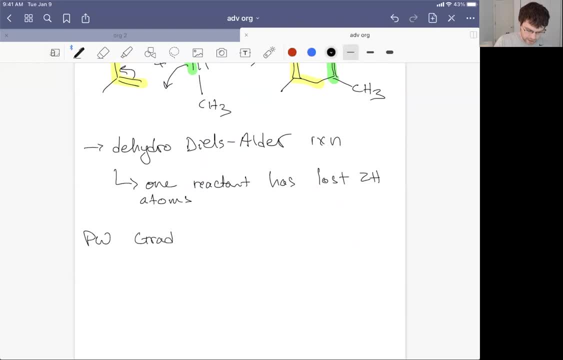 the hexadehydrodeals alder reaction. Now, this isn't- it turns out mechanistically- a true cycloaddition reaction. So I'm going to push arrows that allow you to see what's going on here, And I'm going to push arrows that allow you to see what's going on here, And I'm going to. 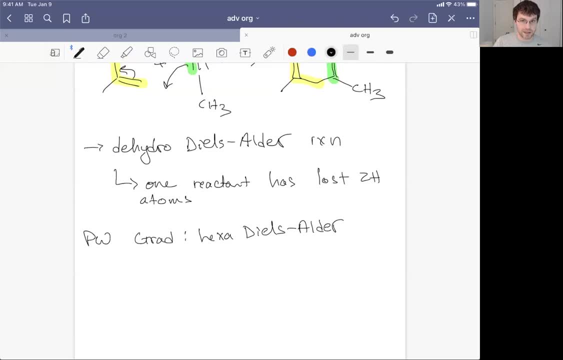 push arrows that allow you to see what's going on here, And I'm going to push arrows that allow you to see what's going on here. But there is a lot of radical character in this mechanism, probably not surprising, given how awkward the structures are. 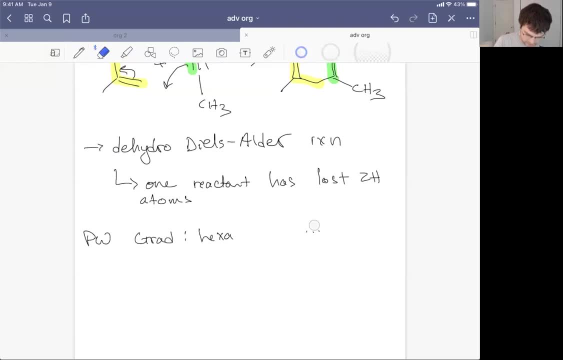 Whoops, hexadeals, alder reaction, Hexadehydro, excuse me. So in this reaction, we're going to, instead of removing two hydrogens to give us the di-dehydro, we're going to remove six. That is, we're going to take our di-ene and remove four hydrogens from it. 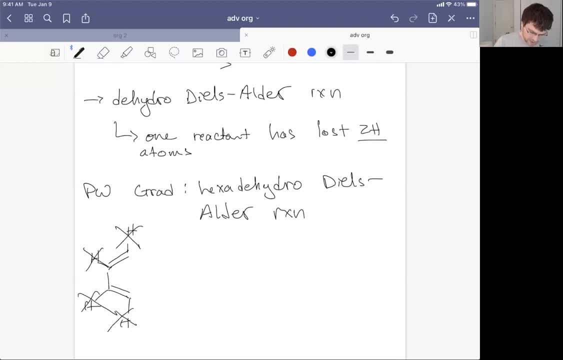 I'm going to cross all of these out and replace them with additional double bonds. That's going to give us a di-ine, a dialkyne, And we're going to add that to an alkyne, which again is like taking our alkyne. 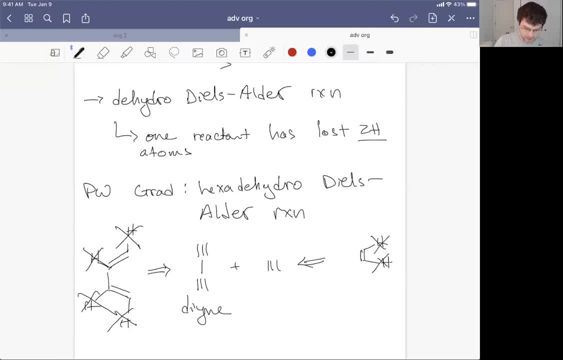 alkene and removing two hydrogens from it to give the dialkyne. Now, when you do this reaction, let's push the arrows again. Imagine these are actually radicals. It allows us to see how things get pushed around. And when you do this, stuff gets weird. First of all, you've got a crazy 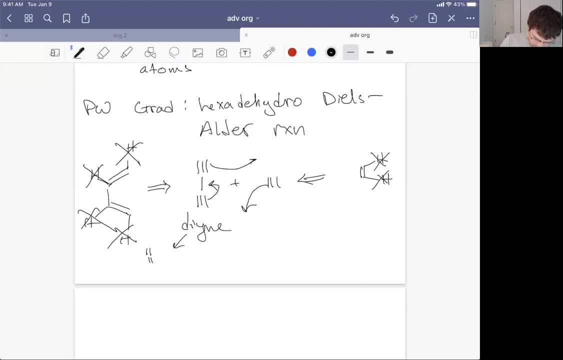 structure that you have to sort of try to relax. So here's our structure. We've got a bunch of double bonds present, but let's go ahead and try our best to relax this into a six-membered ring. So, just like before, we're going to have a double bond all the way over to the right. 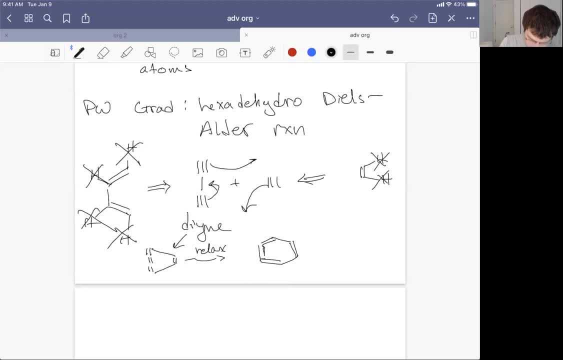 And then now we're going to have double bonds here and then double bonds here. Now this, this is highly questionable at these two positions, because they look as though they've only got two substituents attached to them and perhaps have a lot of sp hybridization character. 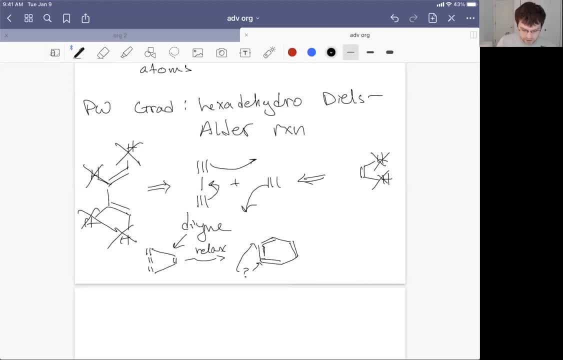 as opposed to sp Two hybridization, which is awkward. Okay, I agree. So what I want to do is I'm going to draw a resonance structure where I roll all of the electrons around. If you think about it, it looks just like how we roll the electrons around in benzene. One of these arrows is a. 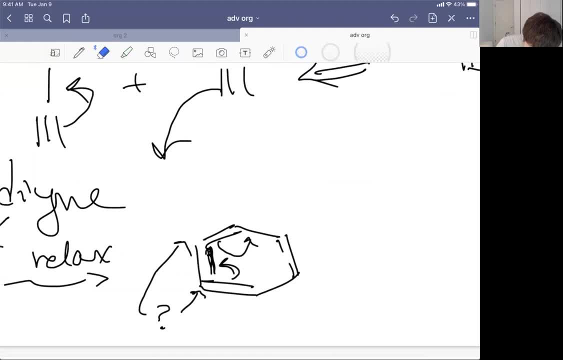 little sloppy and that double bond looks a little sloppy, So I'm just going to clean that up so you can see. All right, So I'm going to go from bond to bond In every case. Now when I do that again, I'm considering a resonance depiction. 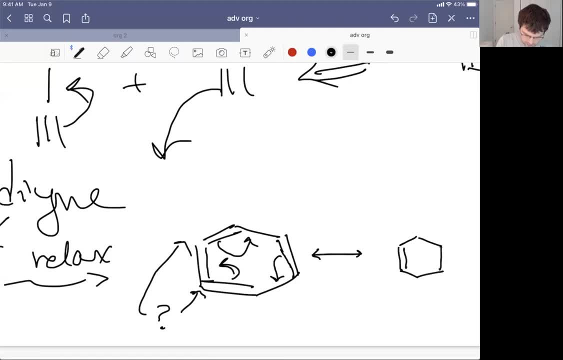 where we now have two pi bonds at the leftmost, carbon and then a typical kind of benzene-like arrangement. Now this overall molecule is near and dear to my heart. This is benzene with an alkyne in it. This is instead benzene. Benzene is a really interesting. 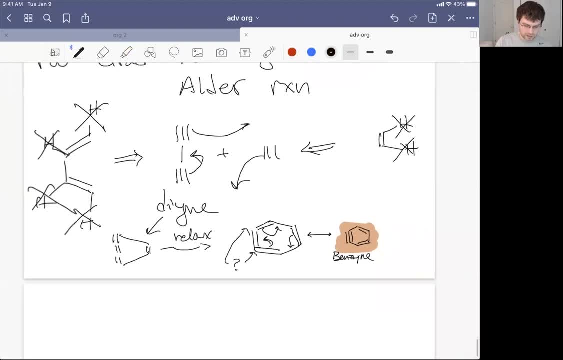 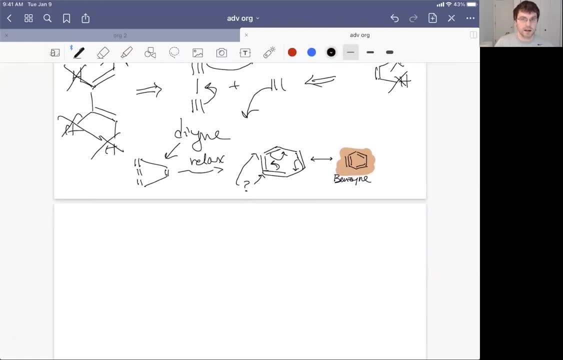 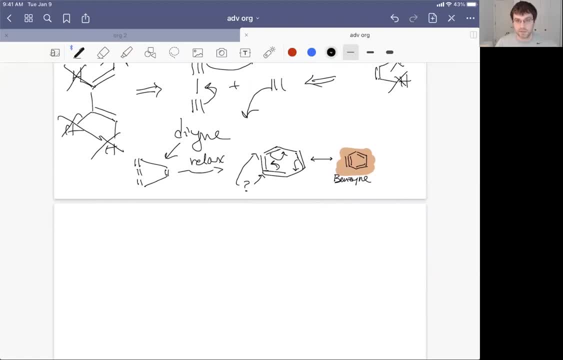 any nucleophile that's on the shelf. Sometimes solvents are not even that compatible with it that we would typically use Additionally. it's a good reactant in a lot of cycloaddition reactions, And so you can even do Diels-Alder reactions on top of this, which is called dominoes. So it's a good reactant in a lot of cycloaddition reactions, And so you can even do dominoes. So it's a good reactant in a lot of cycloaddition reactions, And so you can even do. 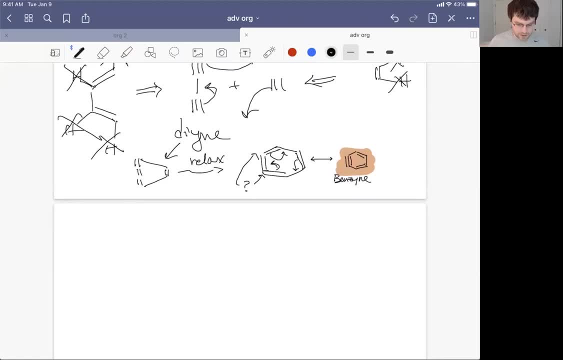 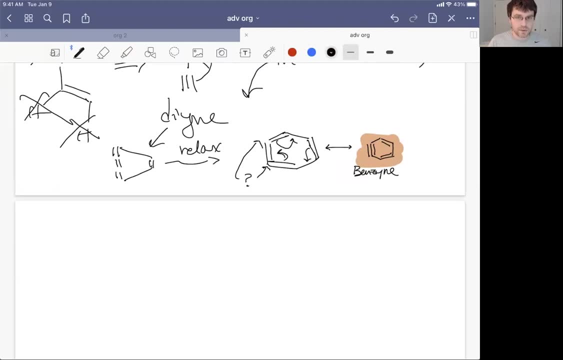 dominoes, So it's a good reactant in a lot of cycloaddition reactions And so you can even do hexadehydrodiels-Alder reactions. So really fun chemistry and I can talk about it in more detail if anyone is interested. Okay, but all of these, well, the hexadehydrodiels-Alder. 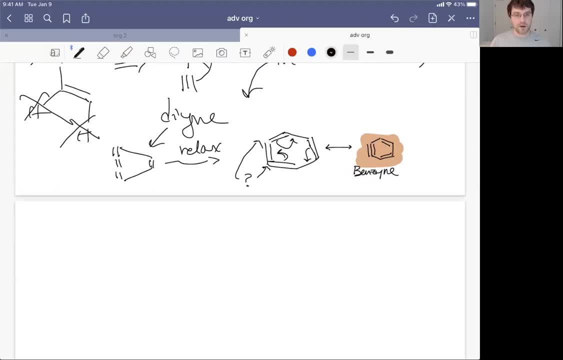 reaction is a bit of an exception, to say the least, But most of these are all sort of four plus two cycloadditions that we were looking at. Are there any other types of cycloadditions? And indeed you could have two plus two cycloaddition reactions. 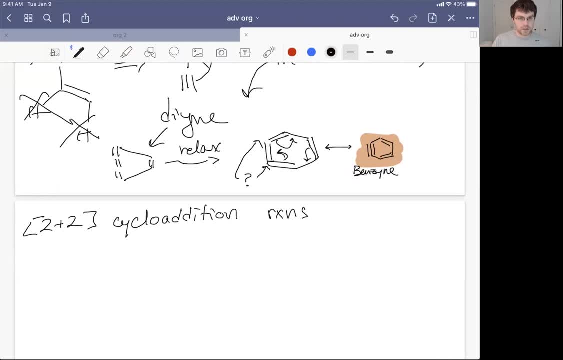 so in two plus two cycloaddition reactions, what you do is you take an alkene plus an alkene, two pi bonded systems and just let them engage with each other. i'm going to draw arrows, kind of going out into nowhere, but it's sort of to show the connection point between the two. 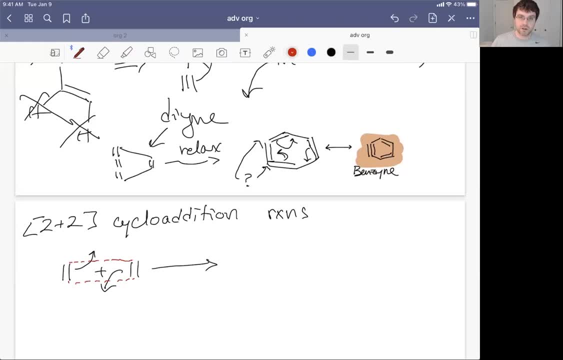 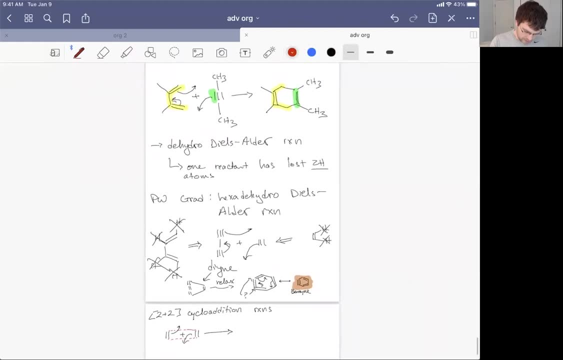 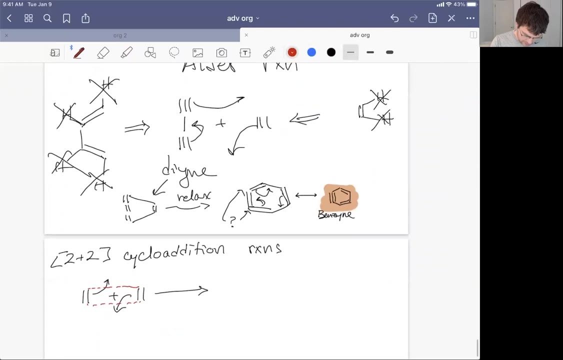 ends of the pi systems. okay, just like sort of how we did the deals alder reaction, but it was a little bit well, not in the hexadehydro case, if we look, if we look up at the top of the screen here, we had those arrows kind of connecting the the termini of the diene to the carbon, the pi, bonded carbons. 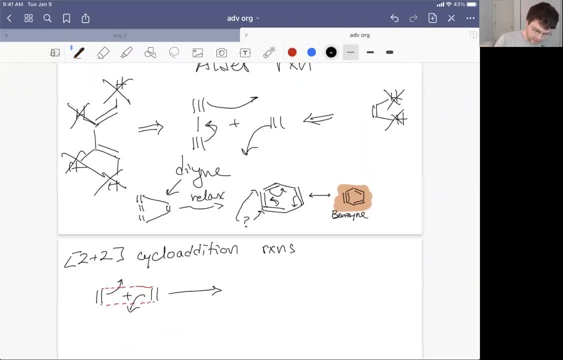 of the dienophiles. we're going to do something similar here and we're going to get a highly strained four-membered ring. so we have our new bonds as part of, in this case, four-membered rings and- and I'm going to go ahead and show you how to do that- 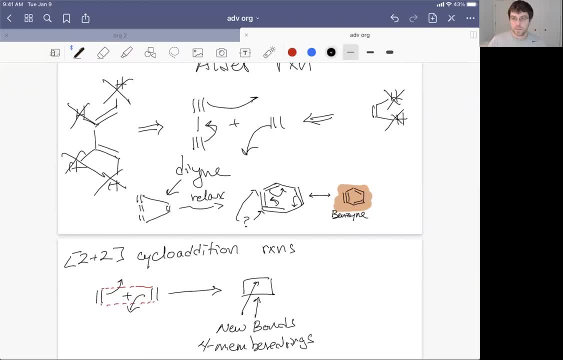 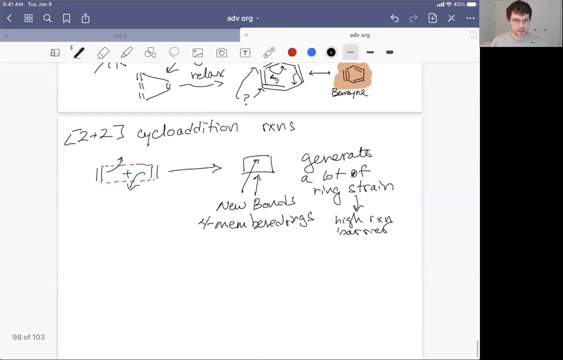 four-membered rings, and so what these do is these generate a lot of ring strain, which means that they require energy input. there's usually a high reaction barrier or activation energy, so I could more precisely say so you have to do some special stuff to get this to actually work. so, um, and if you want to use, to use regular. 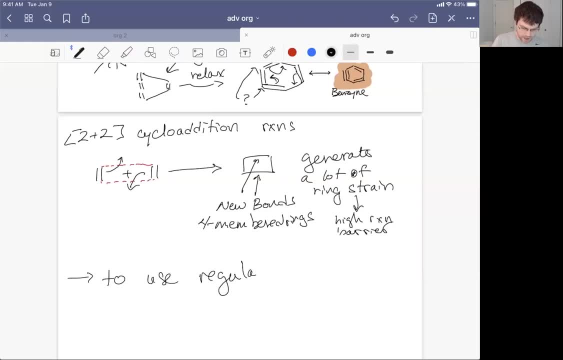 alkenes, just like a typical carbon carbon double bond. um, you need to apply photochemical conditions. it's kind of a weird word. photochemical conditions. let's just say photons are the energy source, and it's not a weird word at all, because we've talked about using h new. 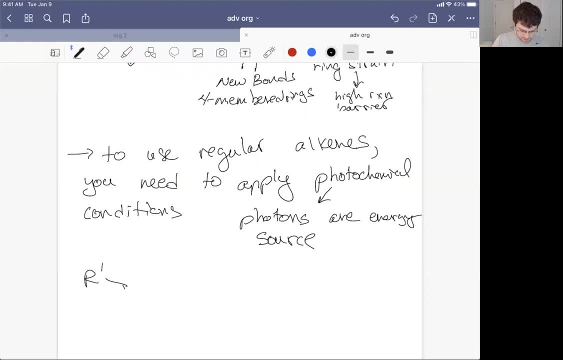 a lot in class. so what I'm saying is is, if we have some sort of alkene with some r groups and let's go ahead and make it z, and we've got r2s over here for another alkene, that's also z. what I'm saying here is: you could apply h new to this reaction and form. 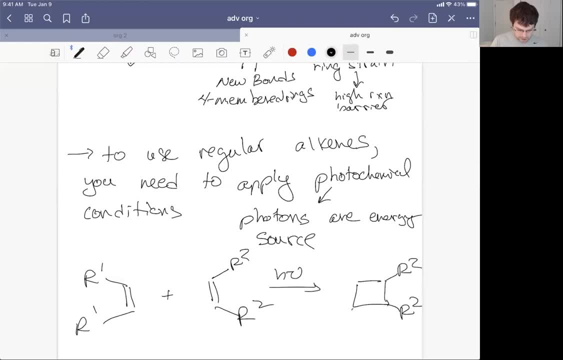 the two plus two product. now, just like the Diels-Alder reaction, it's a little. or the hexadehyder deals all the reactions a little bit. disingenuous to draw the arrows connecting with each other like I've done at the top of the. 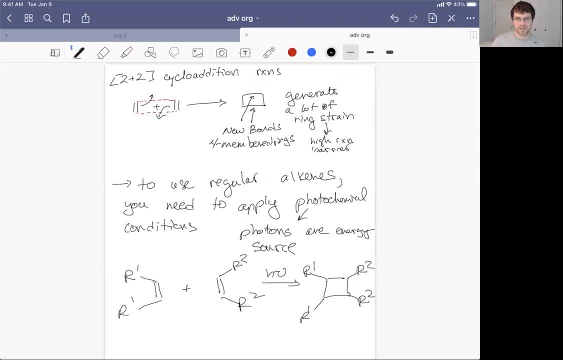 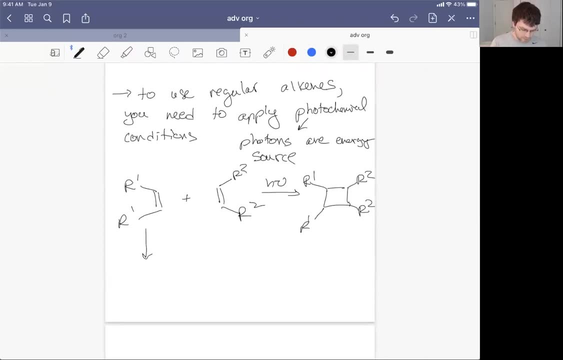 page um here, and that's because this reaction has a lot of radical character with it. now, in many cases, what happens is is that one of the alkenes gets excited by the h, new and the pi bond electrons separate into a biradical system which can engage with the. 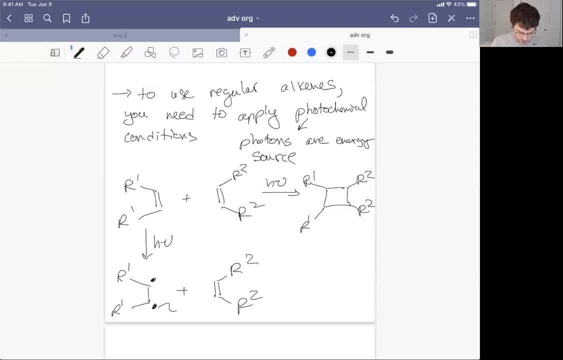 second, alkene. typically if these things are different, one absorbs a little bit better or can kind of take on the energy of the photon a little bit easier. so then we have a radical adding to a pi bond where it splits the pi bond and it's a little bit easier to. 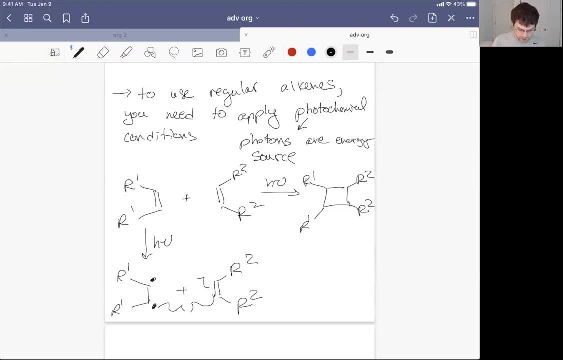 make a new bond which is down below, and then the pi. the other pi electron that was once part of the double bond is now on the carbon that didn't form a new bond but that's now in close proximity to the first carbon that had a radical from the photo photon. 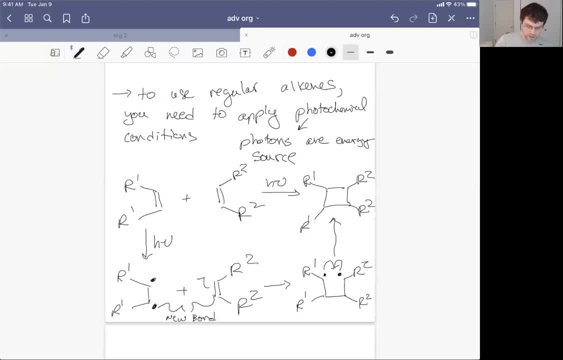 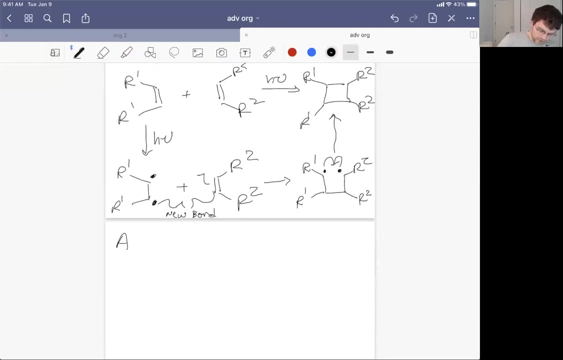 we have a new bond in the top and the bottom to generate the ring system. so that's one approach to doing the two plus two cyclo addition um. alternatively, you can use um some sp hybridized containing uh, carbon, containing alkenes. okay, so let's go ahead and move right into. well, we'll capture that thought, but then we'll move. 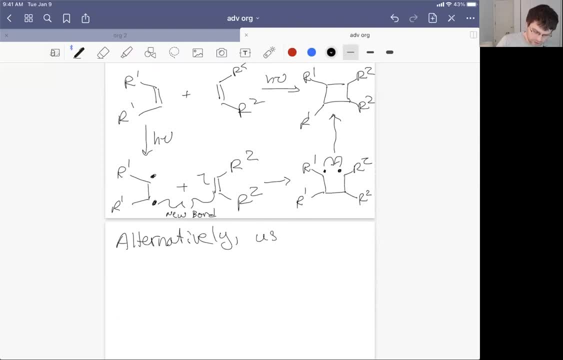 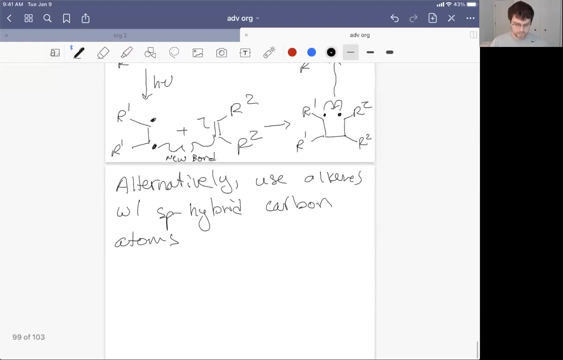 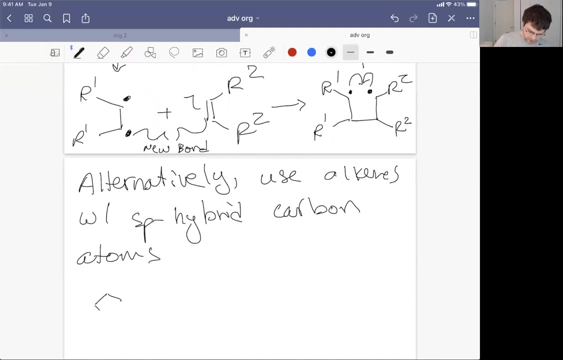 right into some pictures. so, alternatively, we have a new bond and we're going to create a new bond, use alkenes with sp- hybrid carbon atoms, and so what that looks like is, let's say, we take our just a run-of-the-mill alkene, put it inside a five-membered ring. 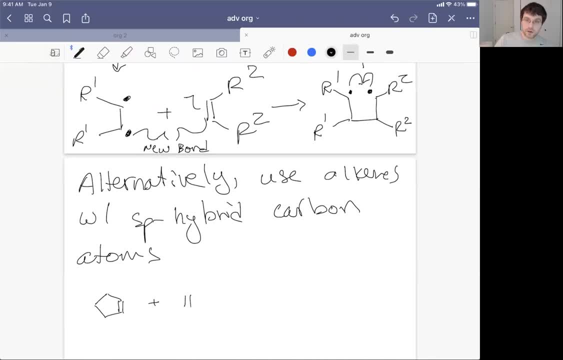 we're going to add that to another alkene, this time under thermal conditions. but we're going to make that that other alkene have an sp, hybridized carbon atom. so typically you would use a ketene. so ketenes, we've looked at an organic two. these were intermediates from the dehydrohalogenation. 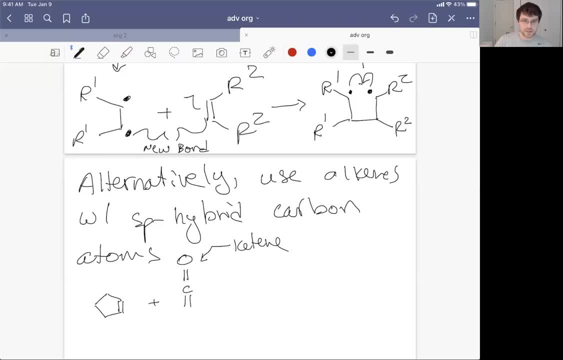 of acid halides, which was towards the end of the semester. so they're pretty easy to make. you just take some sort of acid chloride carbonyl with a sp hybrid carbon atom and you're going to add that to another alkene, this time under thermal. 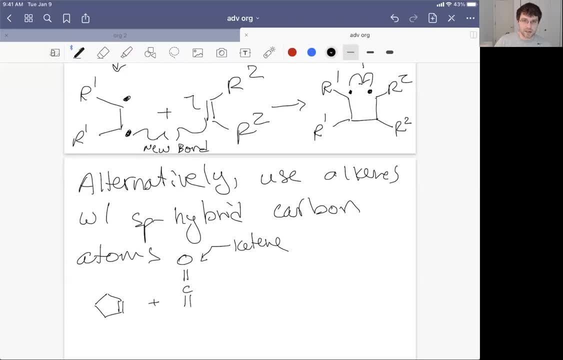 conditions with a chlorine attached to it, treat under basic conditions to eliminate hcl and form a carbon carbon double bond on on a carbon that also has a carbon oxygen double bond. okay, so this is a ketene carbonyl alkene. i guess a ketone alkene. i think that's where the name comes from, or you can.